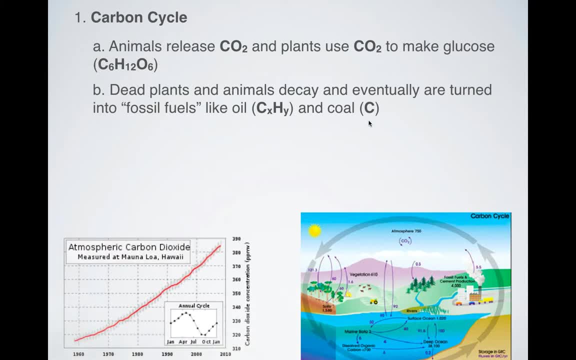 That would be something like oil or coal. Now, when those fossil fuels are burned in the future, that releases CO2 into the atmosphere. And then when that mixes with water through a process that we talked about already called carbonation, that can form carbonates. So carbonates have this. 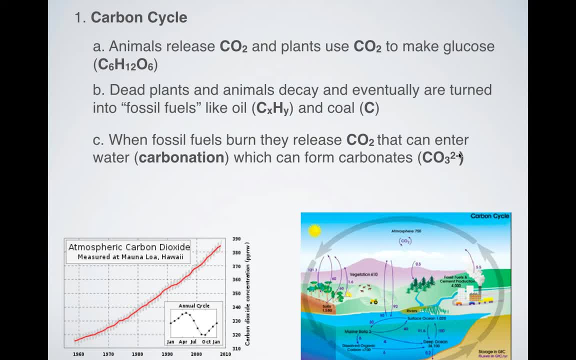 structure: CO3 with a two minus. Now don't worry about the negative signs up here. Instead, just focus on the actual elements. So we've got one carbon and we've got three oxygens in a carbonate. Carbonates are found all over the place. They're found in rocks. 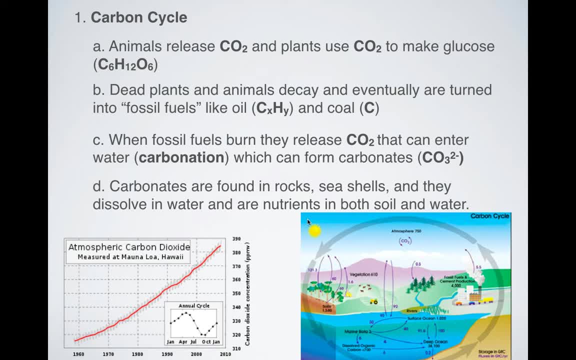 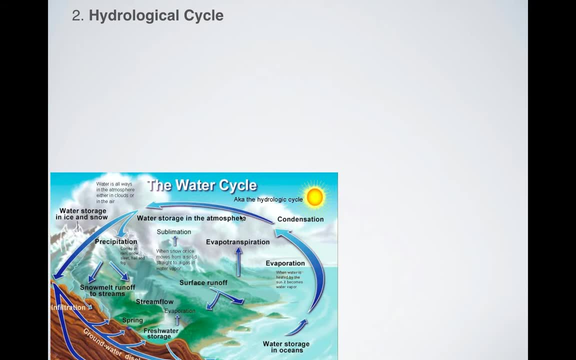 shells. They dissolve really easily in water and they are nutrients that are found in both the soil and then also in water. Now our next cycle, the hydrological cycle, also known as the water cycle, is extremely easy. right. Water is stored in clouds, the ocean, rivers, glaciers. It's stored. 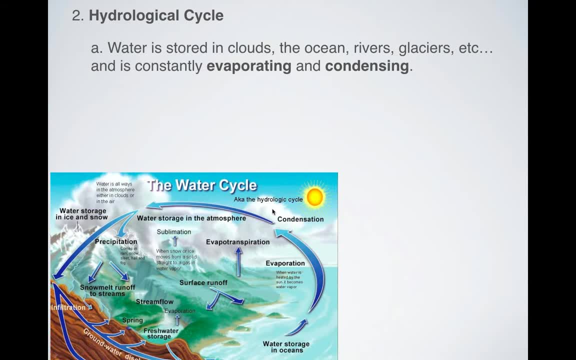 all over the place and water is constantly evaporating and condensing. Evaporation is when we go from a liquid into a gas, okay, And then condensing is when we go from a gas into a liquid, And so when you know like rain happens, 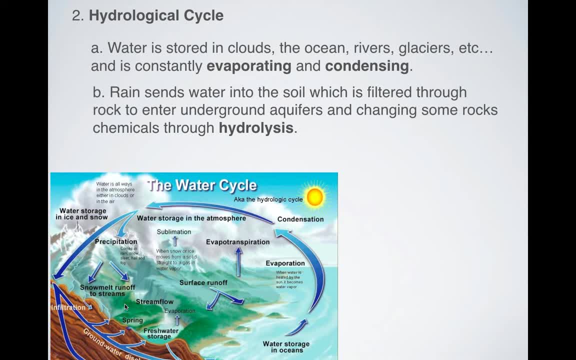 some of that rain is going to land on actual soil. It's going to get filtered, It's going to infiltrate the soil. It's going to go underground into aquifers, which is where we get most of our water from anyway, And then also, you know, we've got some hydrolysis. that's going to happen. 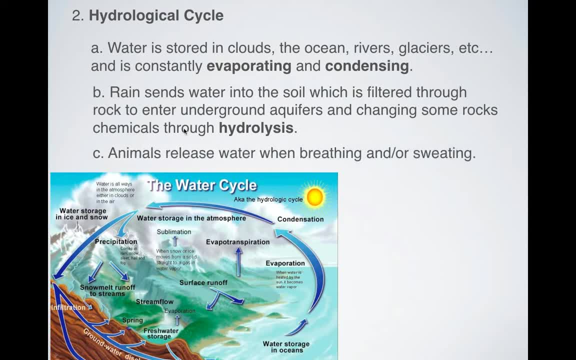 which is a form of chemical weathering that we talked about earlier. Animals will release water when we breathe and also when we sweat. Plants will absorb water through their roots, But also something that not a lot of people realize is that plants also release water through their leaves. 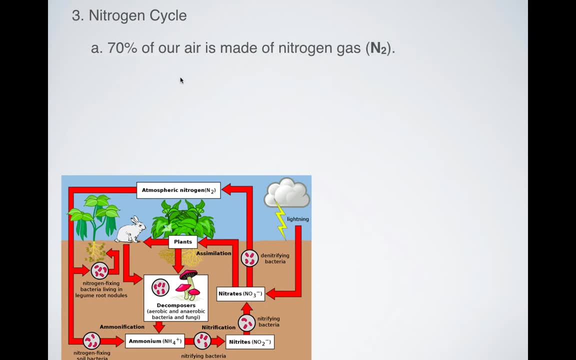 when they breathe. Now, what about the nitrogen cycle? So the nitrogen cycle? 70% of our air is made up of nitrogen. Most of it's not oxygen, It's mostly nitrogen. Where did that nitrogen come from? Well, for the most part we have bacteria called denitrifying bacteria that we find in the 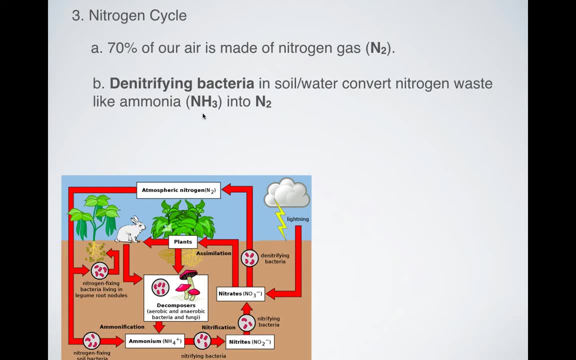 soil and in the water. that turns nitrogen waste like ammonia- which is NH3, into nitrogen gas, which is in our atmosphere Now. nitrogen fixating bacteria and algae will convert that nitrogen gas in our atmosphere into nutrients in the soil like nitrates and nitrites. 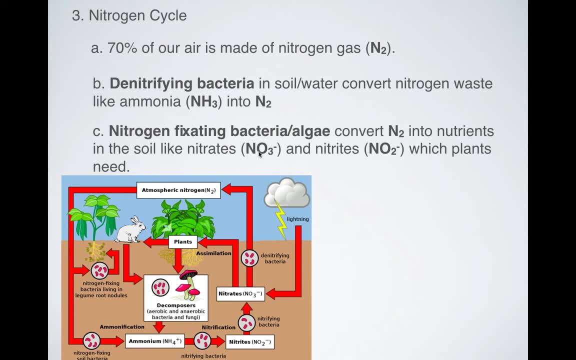 Now again, nitrate has this symbol. Nitrite has that symbol. Don't worry about the negative signs. Instead, just focus on the elements. So we've got nitrogen and three oxygens Here. we have one nitrogen, We have two oxygens. Now, animals, we produce tons of nitrogen, waste right. So it's. 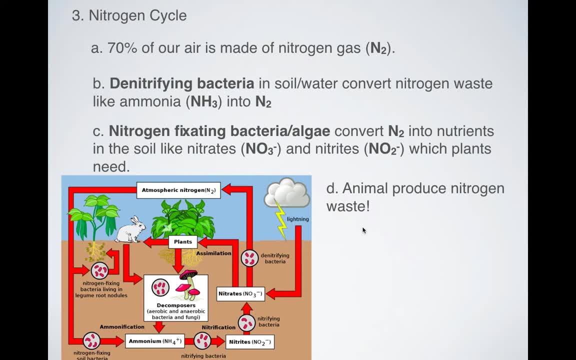 not ammonia that we produce. We produce urea, which is where urine gets its name, But it's the same kind of thing. It's a nitrogen-containing compound. Nitrogen compounds are found all over the place. They can be found in rocks and they can be broken down by abrasion. 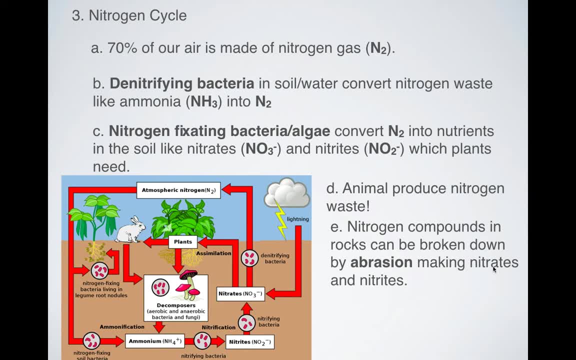 And remember that's a form of weathering that we talked about making nitrates and nitrites go into the soil directly, And something interesting is: lightning has enough energy to turn nitrogen gas in the atmosphere directly into nitrates and nitrites when it mixes with water in the 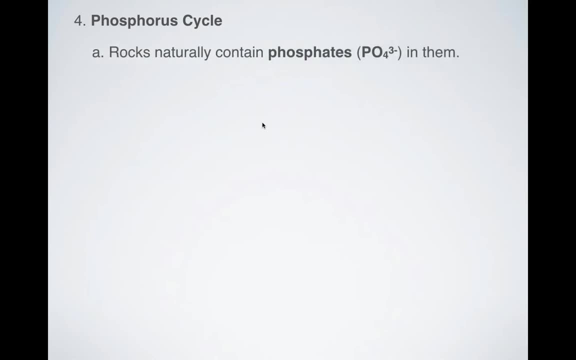 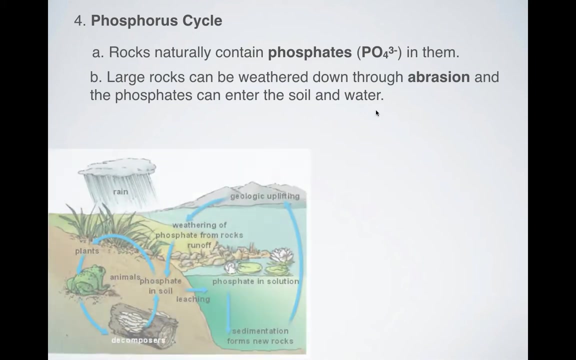 atmosphere. Next cycle: the phosphorus cycle. So phosphorus Rocks naturally contain phosphates. Phosphate has this symbol, PO4, with a three minus Again, just focus on this. We have one phosphorus cycle And we can see that phosphorus and phosphorus are taking a certain amount of phosphorus. 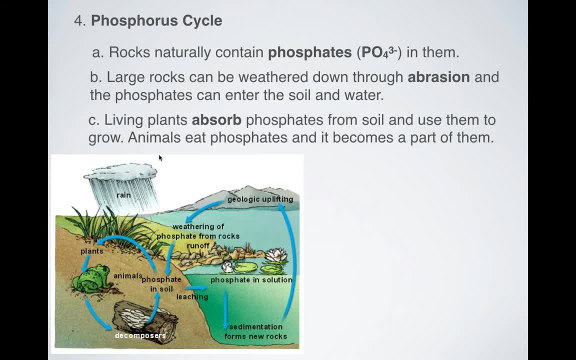 And then phosphorus and phosphorus are also coming back in and they're going to be together down by abrasion and phosphates can enter the soil and the water. Another kind of interesting thing about that is that living plants absorb phosphates from the soil and use them to grow, And then when we 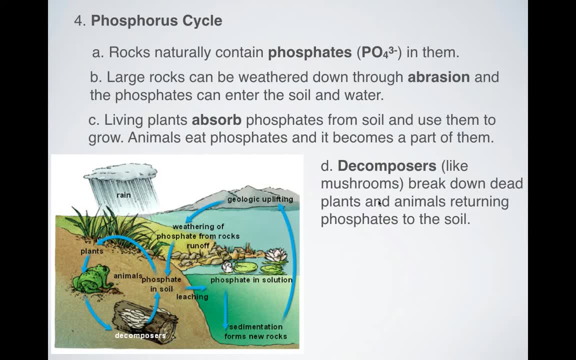 eat those plants or when we eat anything that has phosphate in it, it becomes a part of us and our cells Decomposers like mushrooms. so that's supposed to be like a mushroom break down dead plants and animals and they return the phosphates that were in the plants and in the animals back. 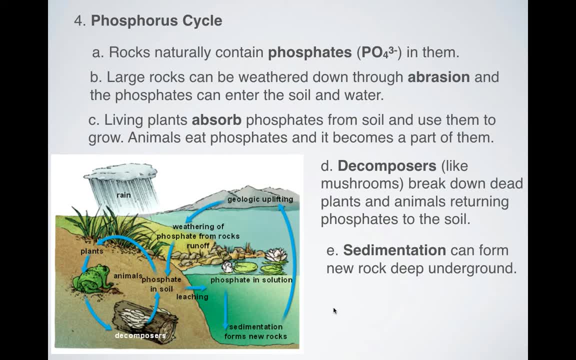 and then they can form new sediments, which would then make new rocks eventually. And then new rocks can be lifted up through geological uplifting, except that would be like the process of making mountains. That takes a long, long time. but the phosphates then can be weathered down again. 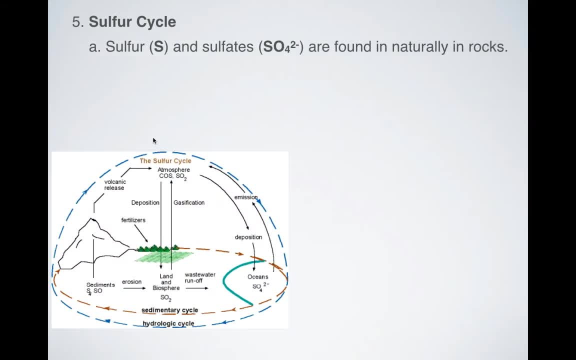 and the process repeats. Last one, the sulfur cycle. Sulfur and sulfates are found naturally in rocks. Again, sulfates have this symbol SO4 2-. but just focus on. we have one sulfur, we have four oxygens. 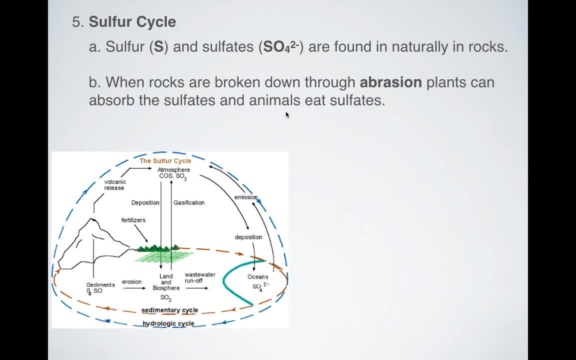 When rocks are broken down through abrasion, plants can absorb those sulfates and animals can eat them also, just like in the phosphorus cycle, right, Except now we're looking at sulfates. Bacteria can consume dead plants and animals putting sulfates back in the soil.